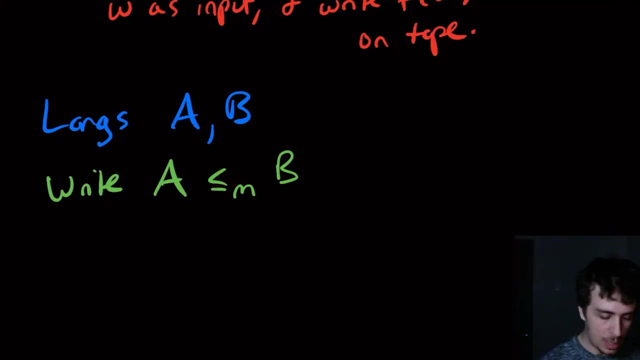 So the m means mapping reducible. The less than equal sign in most computer science in this area actually means reducing or reduction of some kind. it's a reduction. So this thing is what is called a mapping reduction, because part of instruction is linking them. So a dash or m is a 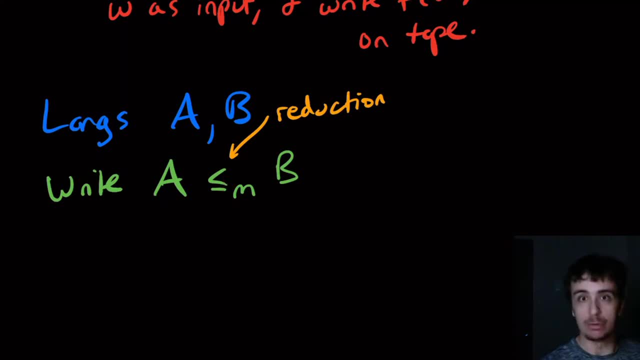 because of what I'm gonna say next. but sometimes, whenever you talk about complexity theory, you deal with polynomial time reductions, and then there you put a P here or a log space reduction, and then you would put an L here, but here is just a mapping reducible thing, and so what? what does it? 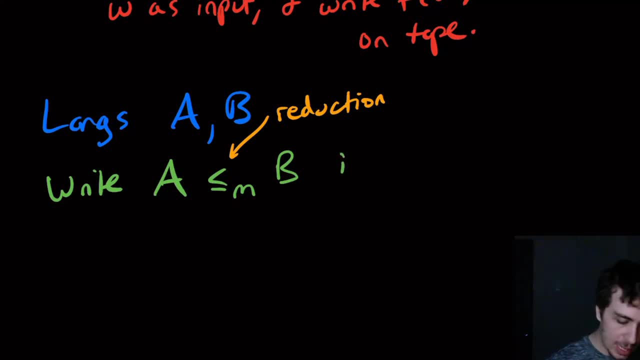 mean to me mapping reducible. so if we're gonna say that this is true, if there is is a computable function, so remember what the definition of computable function is is it can write it out on the tape, so some term machine can write it out. let's call it F, which again goes from Sigma star to Sigma star. it doesn't. 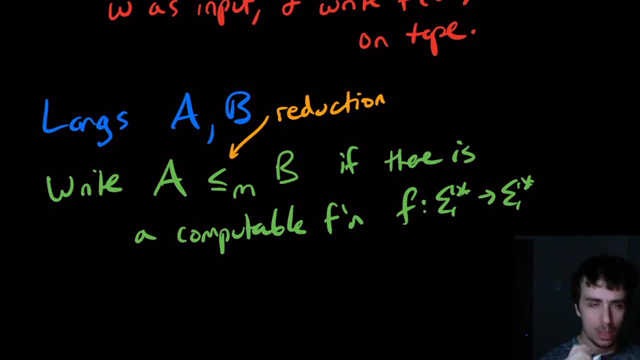 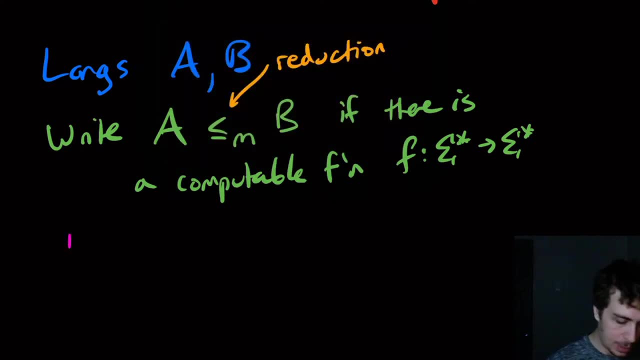 not have to just take inputs from a or produce things that are in B, but there is a certain relationship between a and B. so if there and not if, such that, so if there's a function F such that the following property holds that W in a word, W is just some arbitrary string. if and only 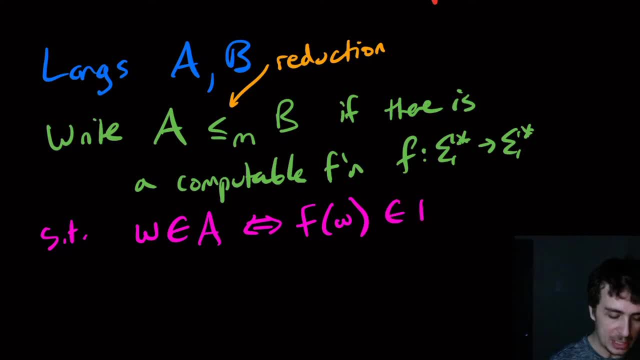 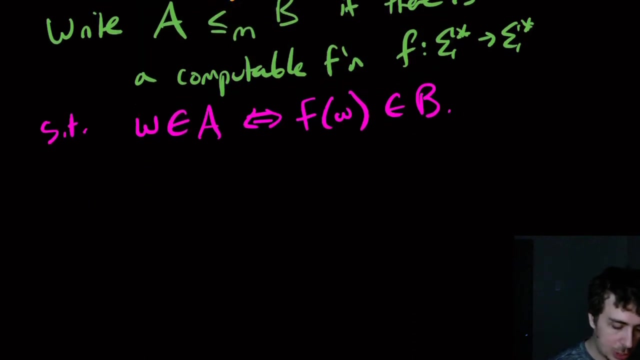 if F of W is in B, okay. so in this sense, the answer of whether the string W is in a is exactly the same thing as whether the produced value, the computed value, is in B. so as an, as an example, we actually saw the following reduction ATM: 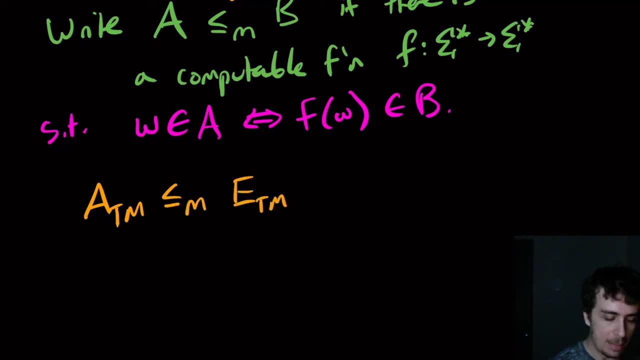 less than or equal to M ETM complement. and why is this? in the proof that ETM is undecidable? we actually what we did is we made a Turing machine and had the prop, it had the property that its language was empty if, and only if, the 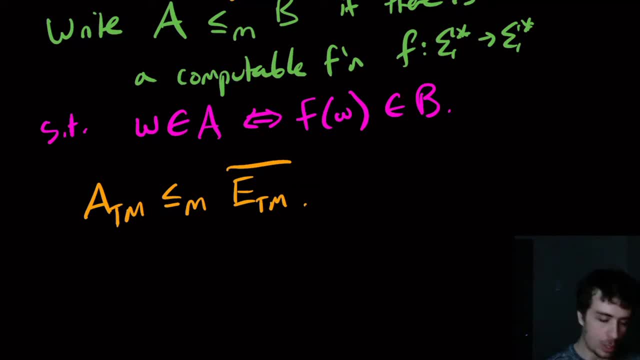 Turing machine M did not accept W, so we had to invert the answer there. so here it was actually a reduction from ATM to ETM complement, because we produced that Turing machine that corresponds to the complement of ETM. so there are some other properties that we're going to show. 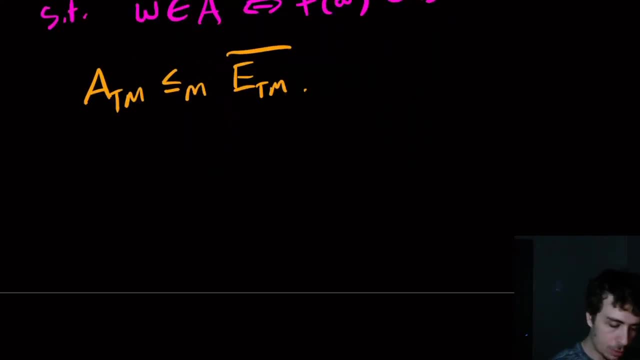 namely this one. so so here's a little theorem that we'll show here, which is that if a oops less than or equal to M, so mapping reduces to B and B is decidable, then a, a, is also decidable, so I don't even need to write out the proof. 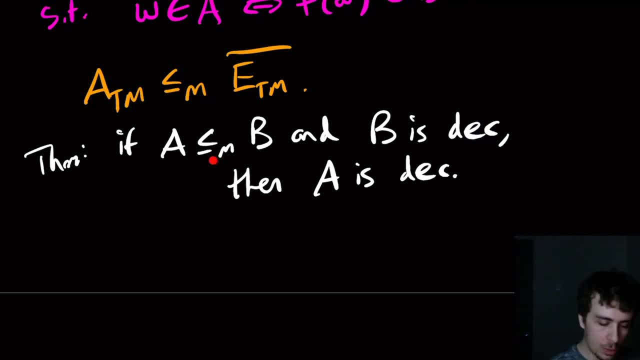 for this, because it's actually very, very difficult to find the proof for this, because it's actually very, very difficult to find the proof for this, because it's actually very, very difficult, straightforward. so the reduction says that there is a function that takes inputs, any old input, and produces any output where the original input is in a 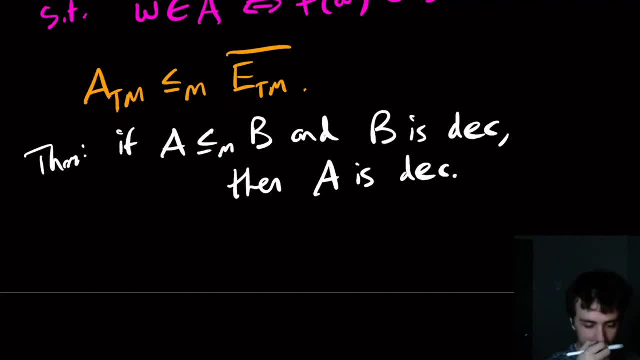 if, and only if, the produced value is in B. so let's think about this. actually, I'll write it out, but I don't really need to. so let's look at this. W is in a if, and only if, the produced value is in B. that's the definition of mapping reduction. so let's let's look at this. if 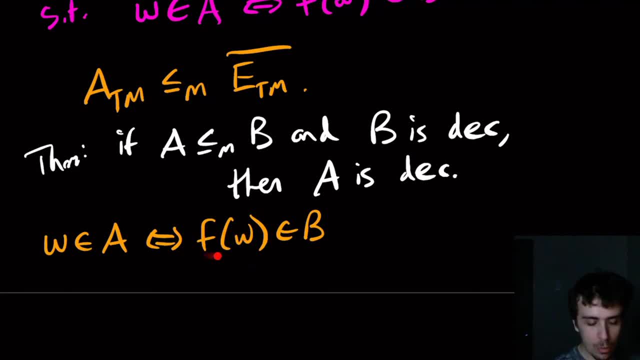 B is decidable, then look, look at what happens. so if we get some arbitrary input- W- and I do not know whether it's an a- I computed the F of W value. it's computable, so it takes only a finite amount of time to produce this F of W. 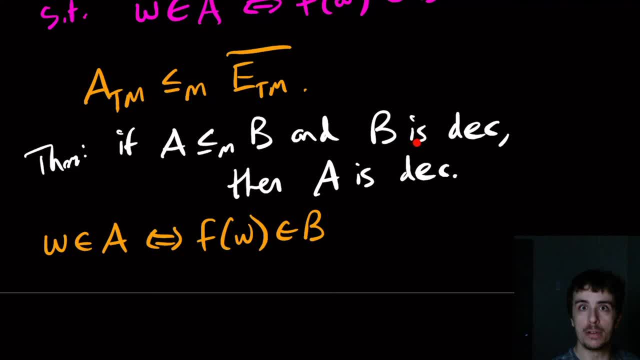 value, then I feed it to the decider for B and then from that, look at this: if B is decidable, then look, look at what this is saying. whatever, the answer of whether it's in B is is exactly the same answer as it is in a, so that means that we can.